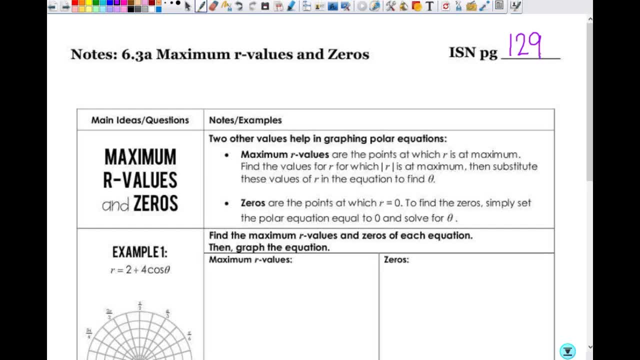 that we have. So it says two other values help in graphing polar equations. So that means, other than the symmetry that we talked about, The maximum R values. what do you think R stands for? Radius are the points where which R is the maximum. 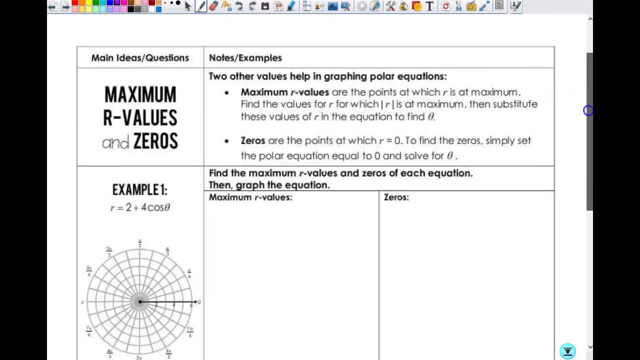 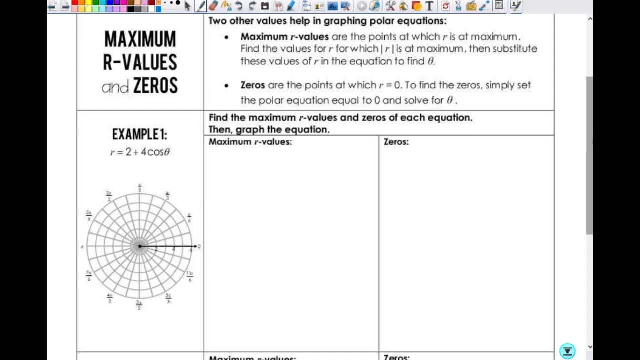 Makes sense, I hope The values for R, for which absolute value of R is at a maximum, then substitute these values for R in the equation to find theta. So the reason it's the absolute value of R is we just care about the distance, and since if I'm at 0 and I have a radius of, 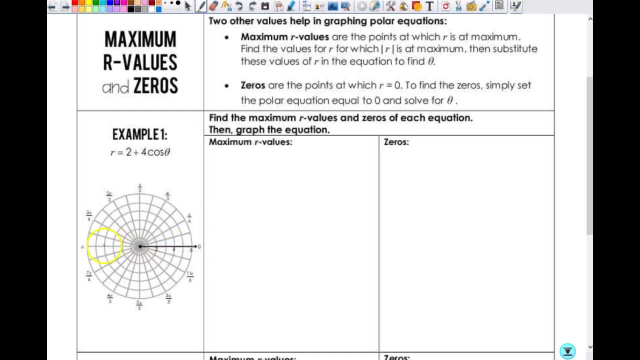 4, I could also have a radius of negative 4 and it'd be over here and you know it still has a distance of 4 from the pole. So that's why we're worried about the absolute value. Then it says: the zeros are the points at which R equals 0. Just 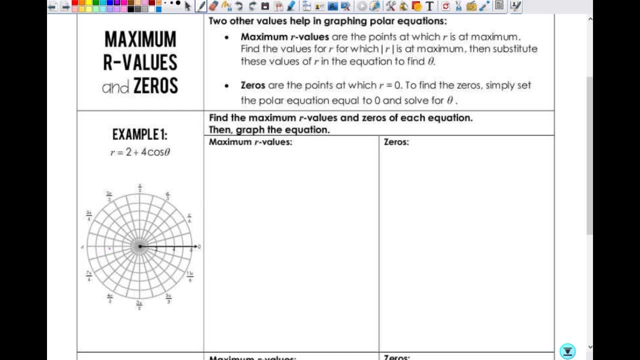 like you know, on the x and y coordinates, when x equals 0. I'm sorry it's when y equals 0. But to find the zeros simply set the polar equation equal to 0 and solve for theta. So same types of things that we have done in the past on. 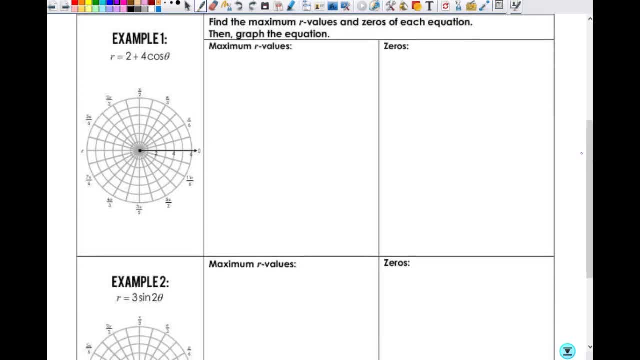 rectangular coordinate systems. And so here this first example. we've got this equation right here. Okay, so we want to find the maximum R values. If I take the cosine of theta, what is the biggest number I can get when I take just the cosine of theta? 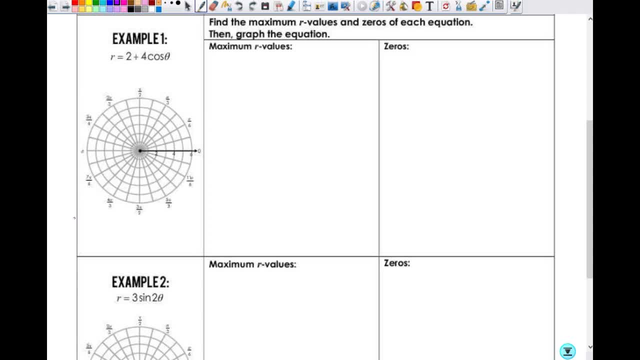 1. and what's the smallest Negative? 1, right, The smallest I can get is negative 1.. The biggest one I can get is negative 1.. 1. That's it. So cosine of theta, whatever it is, has to be less than 1 and greater than. 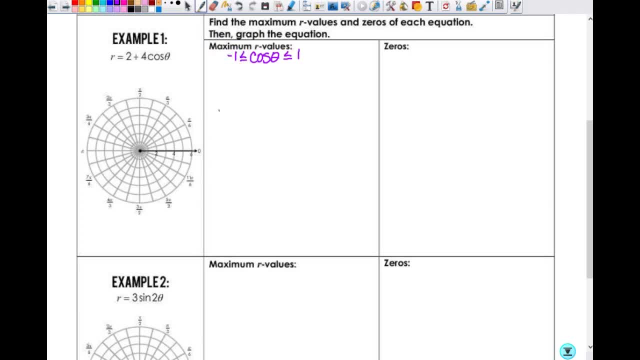 or equal to negative 1.. Make sense? So we're going to look at what happens, since we're worried about absolute value, if cosine theta equals negative 1, right, So then we're going to substitute that into here. Then that would mean that the absolute value of r is equal. 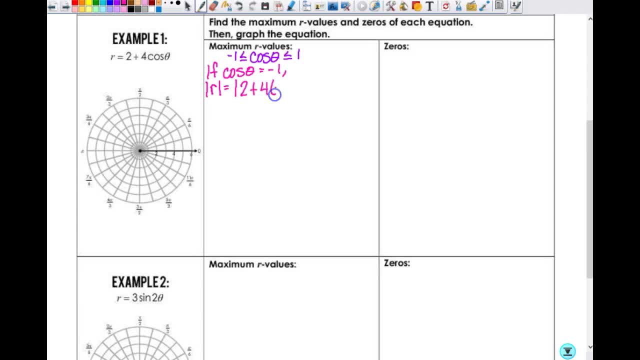 to the absolute value of 2 plus 4 times negative 1, because I'm substituting in that negative 1 for cosine theta, right? So 4 times negative 1 is negative 4, plus 2 is negative 2.. So 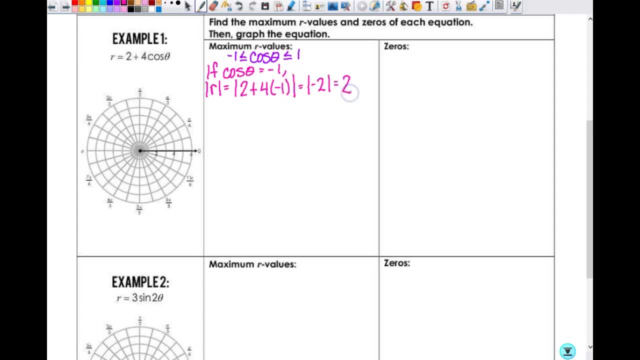 I get the absolute value of negative 2, which is 2.. Okay, Everybody good with that. Then I have to say: all right, well, if cosine theta is equal to 1, then the absolute value of r is equal to the absolute value of 2.. 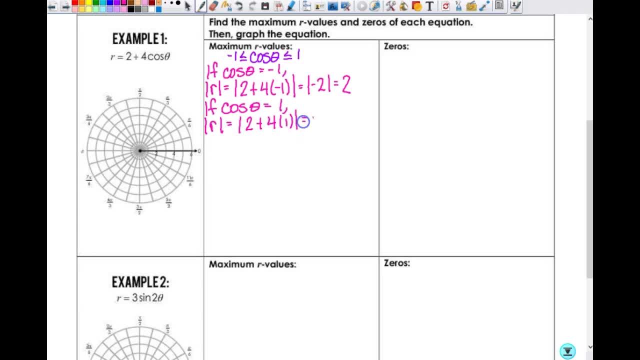 The absolute value of 2 plus 4 times 1 equals. well, 4 times 1 is 4, plus 2.. It's the absolute value of 6, which is 6.. So of those two numbers, which one is the bigger one? 6.. So 6 is my. 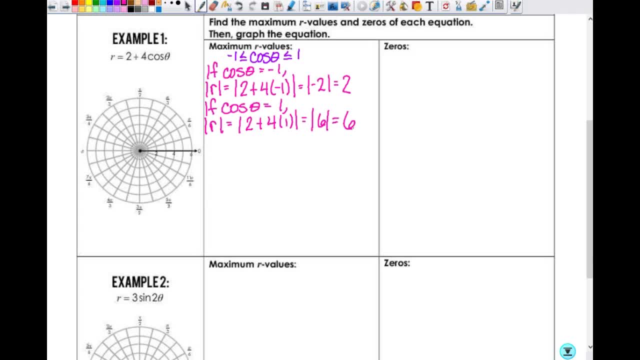 maximum r value: right. But I have to figure out at what angle is that happening. So I actually substitute 6 into this right here, and I get 6 equals 2 plus 4 cosine theta, Right. So then I subtract and I get 4 equals 4 cosine theta, which means 1 equals cosine. 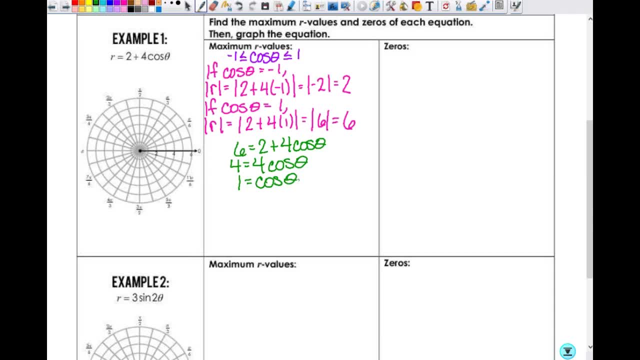 theta. So theta equals what. What is cosine 1? 0 and what? 2 pi. So we're going from 0 to 2 pi on all of these. That's not necessarily the, The, The interval that you would use all the time with these, but you don't know which interval. 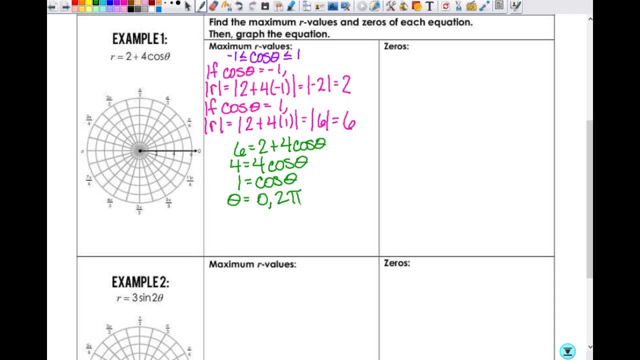 to pick yet. So we're going to go from 0 to 2 pi. That might mean in some cases we have some things that repeat, but for right now that's okay, All right. So then we have to have a final statement here, and our final statement is that the absolute value of r. 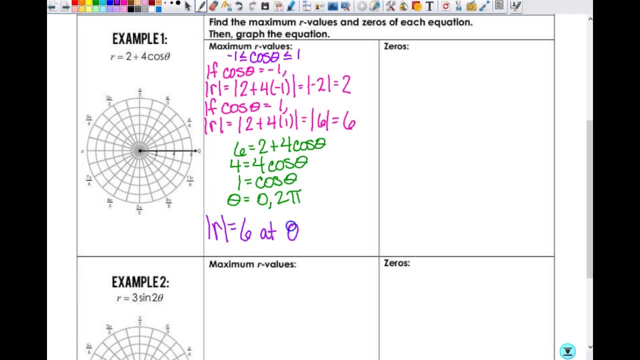 is equal to 6 at theta equals 0 and 2 pi. So that means on my graph here where I'm going to go and plot that, well, at 0, I have a radius of 6, and at 2 pi I have a radius of 6.. So even going from 0 to 2 pi, there's 0 and 2. 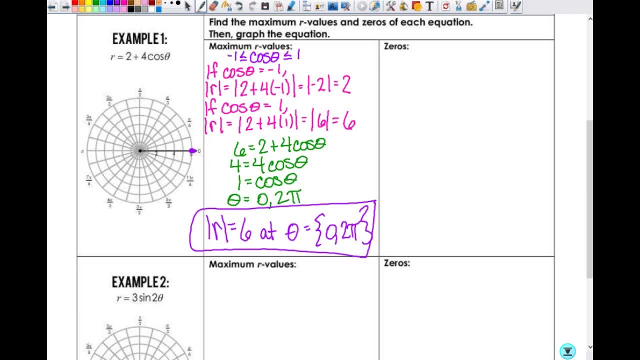 pi overlap sometimes. but there we go. Okay, I also need the zeroes. So that mean I need to know when the radius is 0. So I take 0 is equal to 2 plus 4 cosine theta. So it gives me a negative 2 equals 4 cosine theta. The negative 1, hats off to you. Here we go. So. 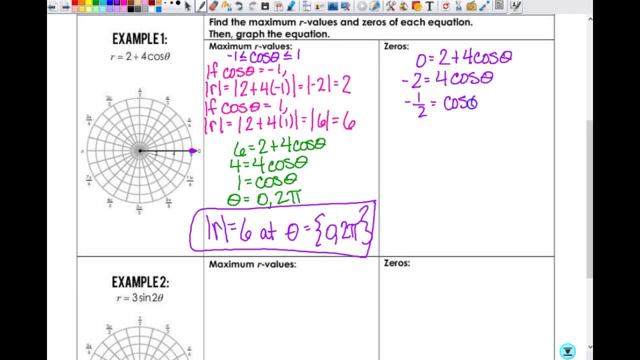 So negative one-half equals cosine theta. So from zero to two pi. when is cosine a negative one-half, Two pi-thirds and four pi-thirds good? So then I say: r is equal to zero at theta equals two pi-thirds and four pi-thirds. 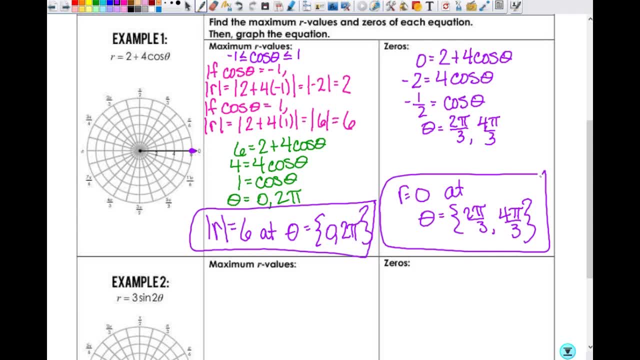 So let's look at how that gets me some help over here on this graph. First of all, I do know that r does equal zero at somewhere, so there's a point there. But when I put that I mean I don't know. 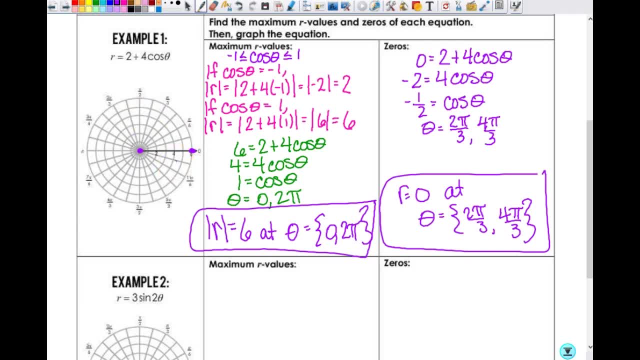 I don't know which angle that's coming from right. That's why I have to find this. So, at two pi-thirds is where it actually hits zero. Well, from zero as an angle, all the way to two pi-thirds, that means there's a radius other than six, well, other than zero, for sure, and other than six. 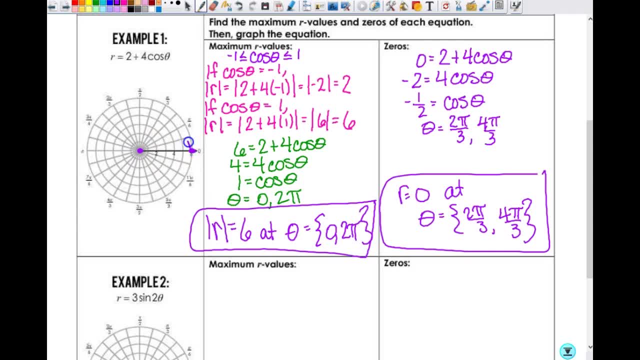 So that means it's going to swing out something like this, Like it's going to start rotating around and then, when it gets to two pi-thirds, it's got to hit zero. That is not good. Let me do that again, Sorry. 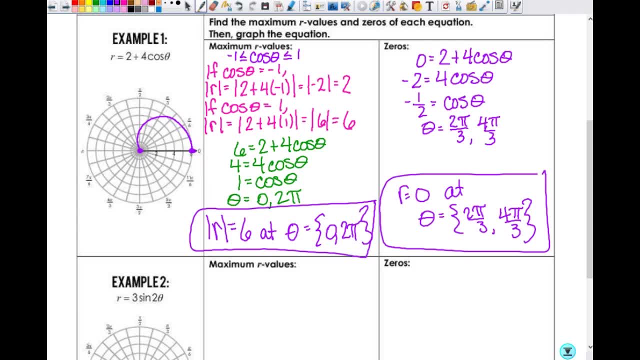 It looks something like that: Okay, where it kind of it's not like a semi-circle, It like comes in and gets a little closer in there, I didn't do that really great. And then the next one's at four pi-thirds right, which means that also happens on this side. 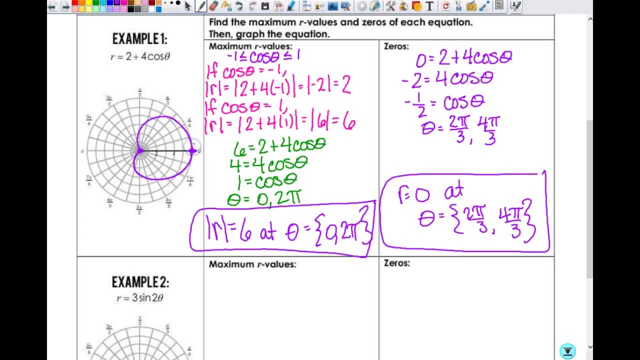 So it comes out something like that Kind of looks like a heart, but it's not pointing down there And these should be. it should be symmetric. I'm not redrawing it again, We're just sketching right now. It's fine. 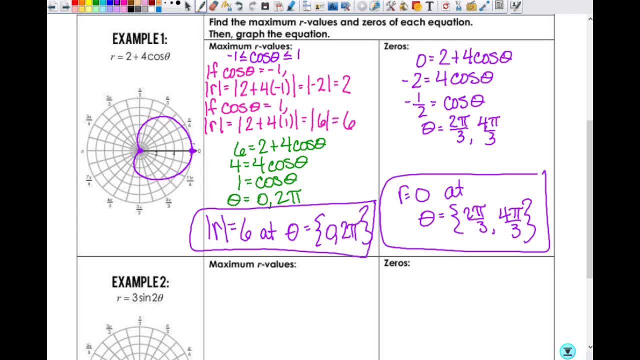 Okay, So we're going to go with that, But it's like a continuous curve. It's not a point like a heart, but it does kind of dimple in right there. Now in this case- and I again I know you don't know a whole lot about these graphs- 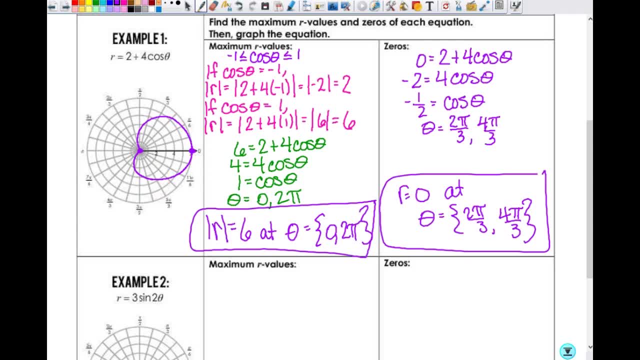 So on the assignment, I had actually kind of not put the graphs on there at first, and then I went back and put them because I want you to attempt it. If they're completely wrong, it's fine. I just want you to start thinking about what makes sense with the information that we have. 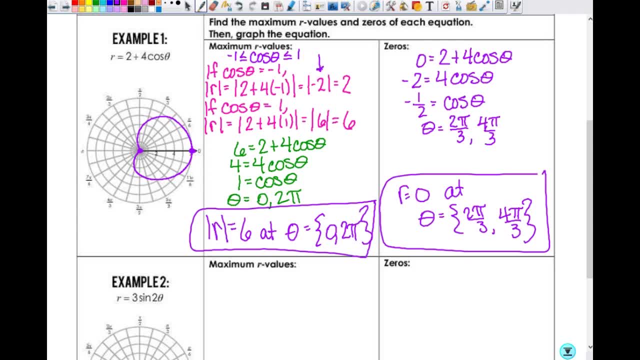 This negative two radius right here actually does give me some information, Like it's an important part of this. It's just not my maximum, So the negative two. if I was to substitute negative two in for r, what I get is pi. 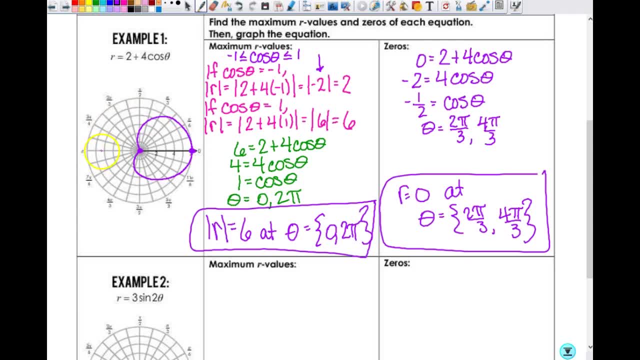 So I'm just going to tell you that without us doing it. So when I go to pi, my radius is negative two, which means I have a point right here. So what this graph actually does is it's when we start at zero. it comes in. it goes like this: 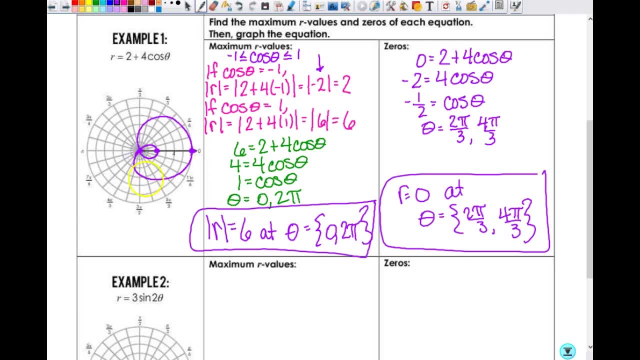 It loops around inside of here and then goes back out that way. Okay, So it looks something like that. Yeah, if you get something that, if you think that you know it's at least the hard part without the loop, I think you can get. 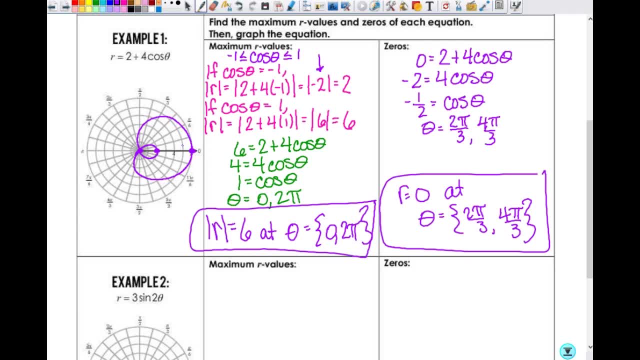 And if you think there might be a loop and if you don't know, it's okay. What I don't want you doing on the homework yet, because we will, I don't want you graphing on a graphing calculator or trying to look at the graph itself. 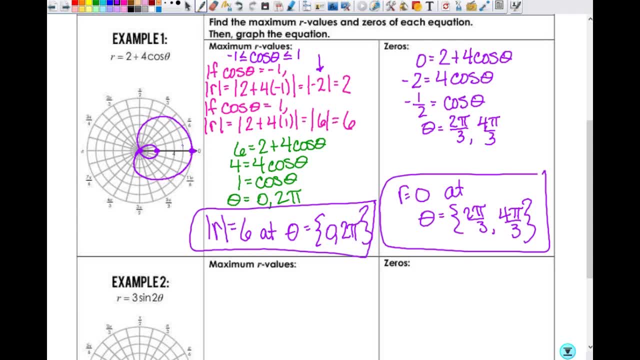 I want you to think about what makes sense to you, and then we will go and like, actually look at some of them that are graphed for us. okay, because it's just going to kind of it kind of spoils what you're thinking up until that point. 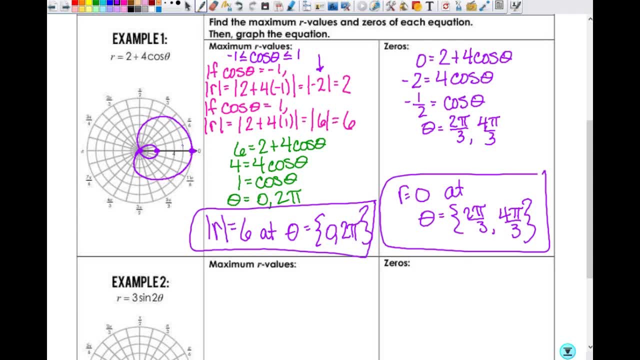 And this one's, as far as you not understanding and going with this, this one's the weirdest one, and there's not all going to be that. they're not all going to be that confusing if you don't know what you're doing yet. 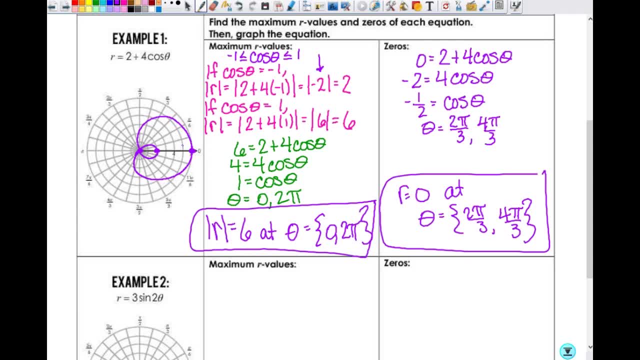 Okay, Are we good so far? We at least understand that part. This is just kind of like a little bonus, let's think through it, type of thing. Okay, We're going to skip number two. We're going to go to number three. 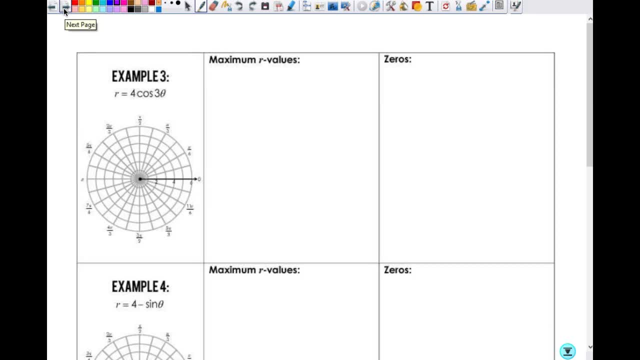 And because I'm skipping some of these? because we don't need to do every single one of them. it just so happens all the examples are cosine There's, that's just a coincidence. I just skipped the sine ones, not because they're bad. 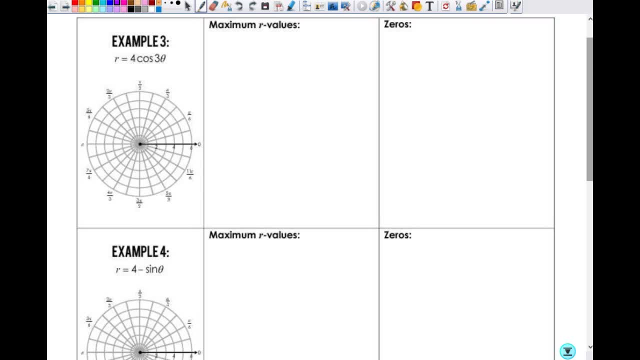 but because, just because I guess that's one I chose, All right, So I'm going to go back to the first one. So I have this equation: now I want the maximum R-value. So now this has cosine of three theta. 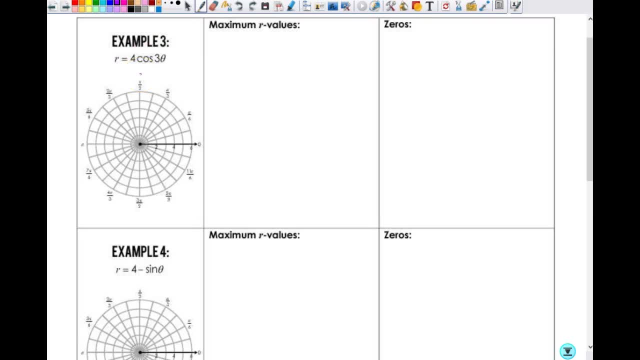 So three theta is just some number. Whatever this number is, when I take the cosine of whatever it is, still the biggest number I can get is one and the smallest one is negative one. So then, now here the cosine of three theta, not just the cosine of theta. 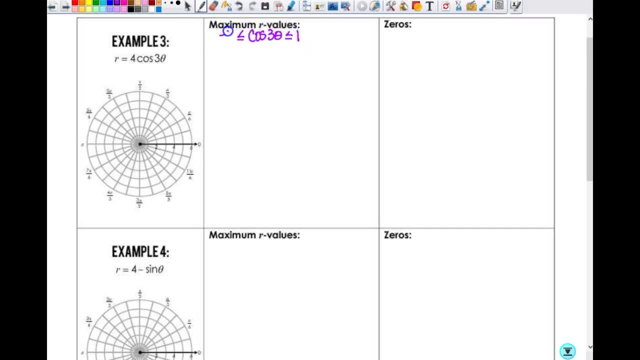 has to be less than or equal to one, greater than or equal to negative one. Okay, So then I say: well, if cosine, theta, cosine, three, theta, sorry- equals negative one, then the absolute value of R is equal to the absolute value of four times a negative one. 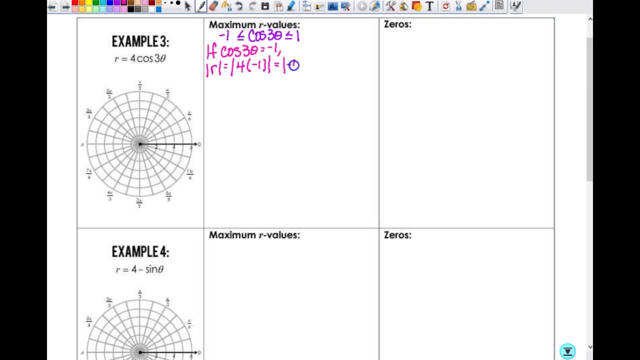 And that's going to be absolute value of negative four, which is four. Right, Then I have to do the positive one. So if cosine three theta equals one, then the absolute value of R is equal to negative one, And that's going to be the absolute value of R equals the absolute value of four times one. 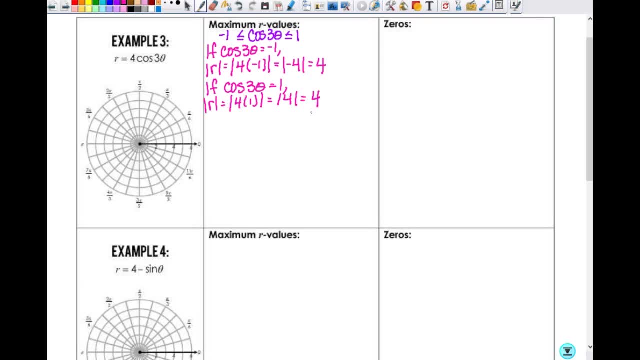 which is the absolute value of four, which is four. So I got the absolute value of R equals four for negative one and one. So when I go back to find the angles I have to use both of them Right. So when I go in here and I'm going to substitute in the negative four, 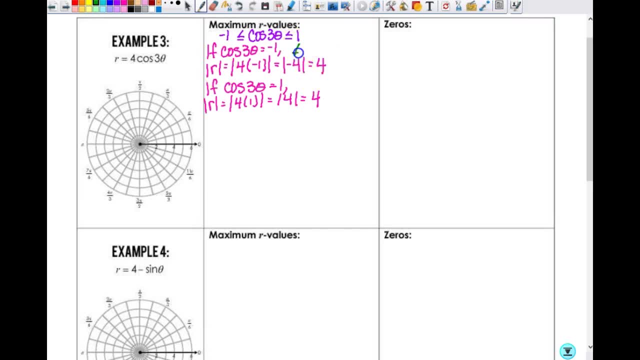 because even though I get a positive four here, for the absolute value the radius here is still negative. So that means that negative four is equal to four times the cosine of three theta. And then I'm also going to use this radius here, which is a positive four. 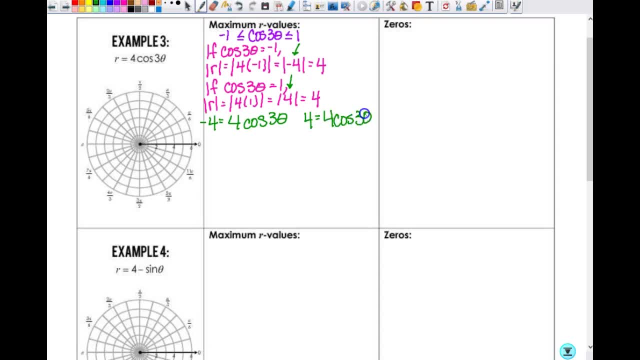 And that's equal to four times the cosine of three theta. And then I have to solve both of them. Okay, So we'll start with this one. I'm going to divide both sides by four, So I get negative. one equals the cosine of three theta. 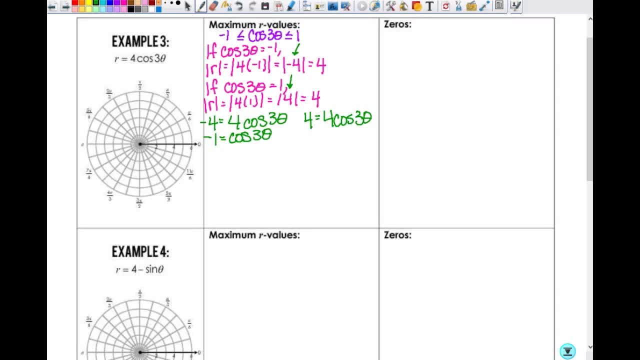 So in order to get that three theta away from cosine, I have to take the cosine of three theta, Cosine inverse of both sides, Right? So what that's going to give me is three theta. It doesn't give me theta yet. 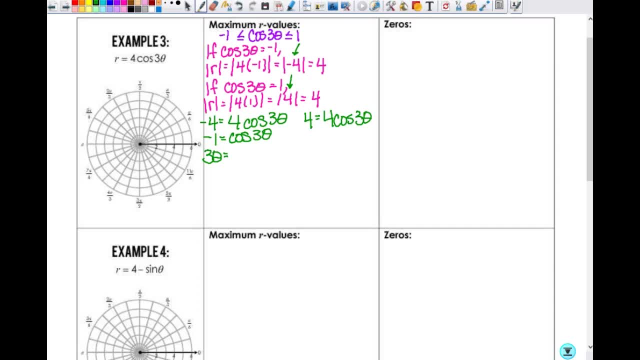 When is cosine negative? one Pi. Okay, Now here's a little part that you have to think through. In order to get theta, I'm going to have to divide everything through by three. Right, My theta has to go from zero to two pi. 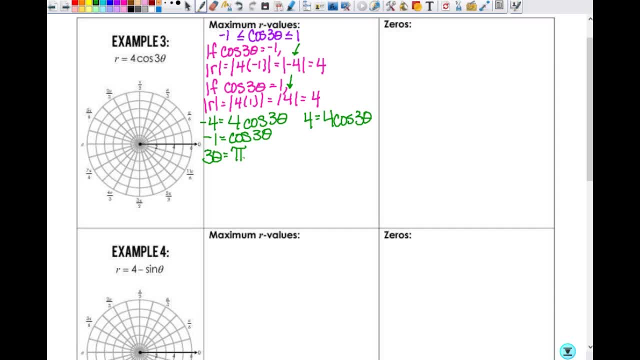 Well, if I'm about to divide by three, in order for me to get from zero to two pi for theta, my three theta has to go from zero to six pi. Does that make sense to you? Because if this is a three, I have to triple my zero to two pi range there. 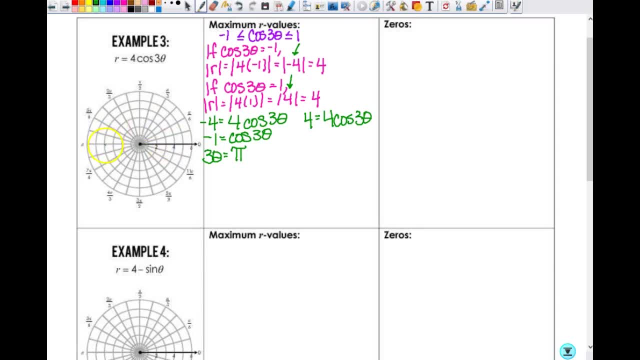 So instead of just pi. so I am here like this is your negative one, It's pi. So this is two pi, This would be three pi, And this would be four pi, And then five pi, And then that would get me through six pi. 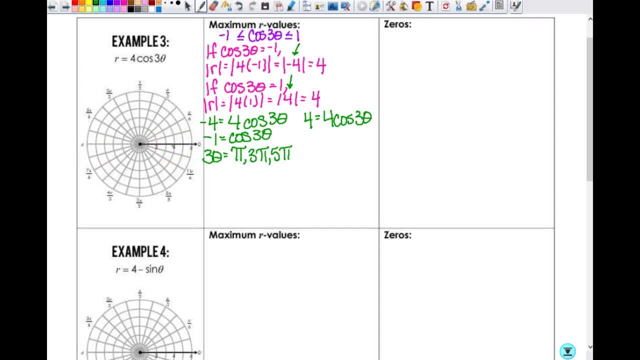 Okay. So If you have something other than just theta, if it's three theta or whatever, that changes the amount of angles you have to have right there. We're used to stopping at two pi, but you're going to have to go farther. 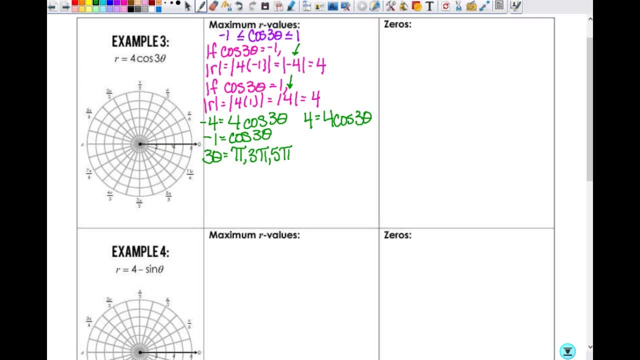 Because now to get theta, I'm going to divide everything through by three And I get that theta is equal to pi thirds. What's three? pi thirds Pi And then five pi thirds. So in the end my theta does go from zero to two pi. 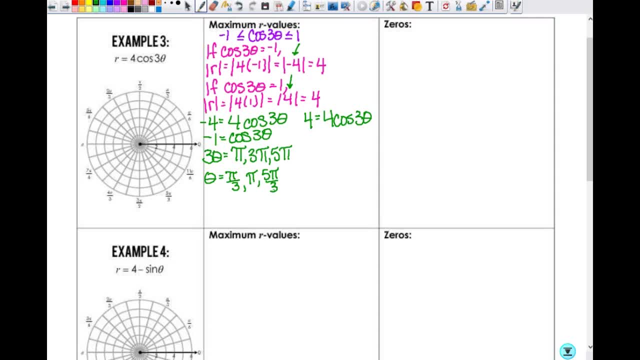 You with me on that. So now I look at four and I solve this one. I get one equals cosine of three theta. So three theta equals Well cosine is one at zero, and then at two pi, and then at four pi, and then at six pi. 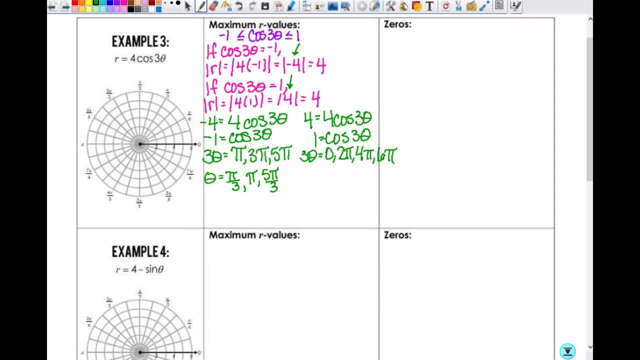 So now, when I divide everything through by three, I get that theta is equal to zero. two pi thirds, four pi thirds. and what? Two pi Bless you Okay. So that's lots of angles there, And that means that the absolute value of r equals four at theta equals. 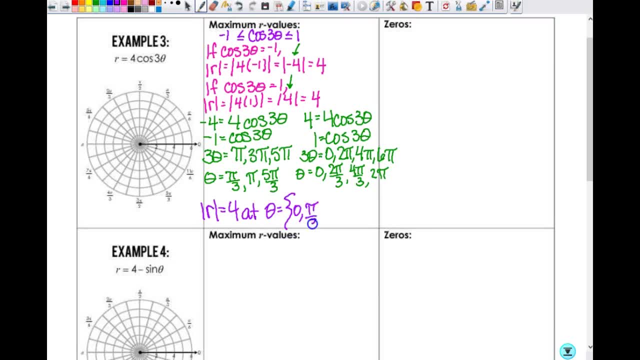 And then we start with zero: Zero pi thirds, Two pi thirds Pi Four pi thirds, Five pi thirds, Two pi Okay, Everybody okay with all that. so far, Let's plot the radius. So here's what we have. 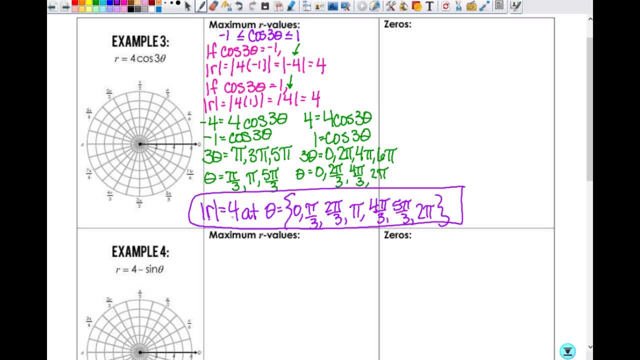 It's the absolute value of four at those. But this, these three right here, came from The radius that is a negative four, And these came from the radius that is four right. So at zero I have a radius of four. 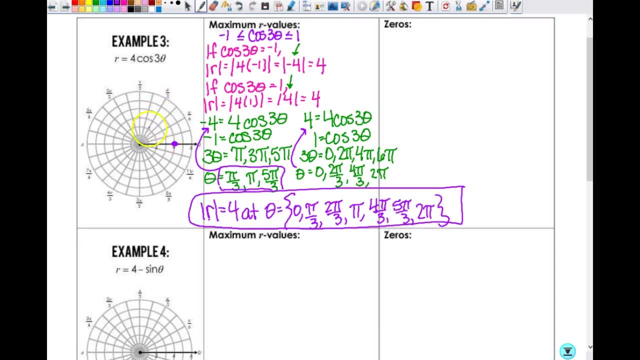 At pi thirds, my radius is negative four. right here, At two pi thirds, my radius is four. right At pi, My radius is negative four. I already have a point there. At four pi thirds, which is right here, my radius is four. I already have a point there. 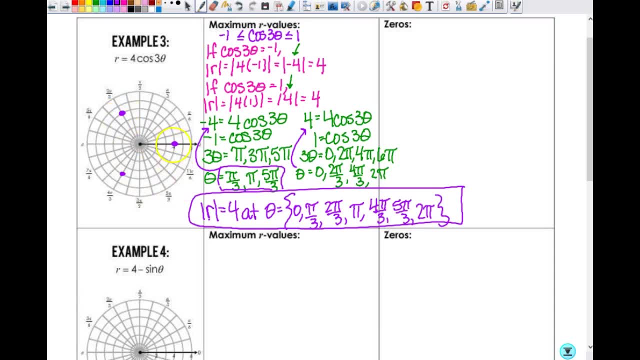 Five pi. thirds: it's negative pi- I already have a point there. Two pi- it's four. I already have a point there. So we end up repeating there because we didn't really need to go that far, but we didn't. 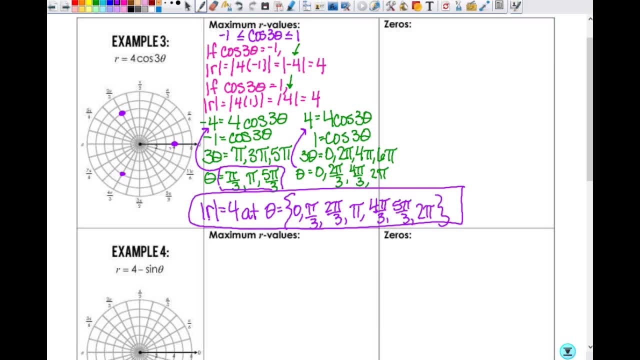 know that right now. Okay, We good so far, All right. Now we gotta find the zeros. So zero is equal to four times the cosine of three theta. That means I divide by four and I get zero equals the cosine of three theta. 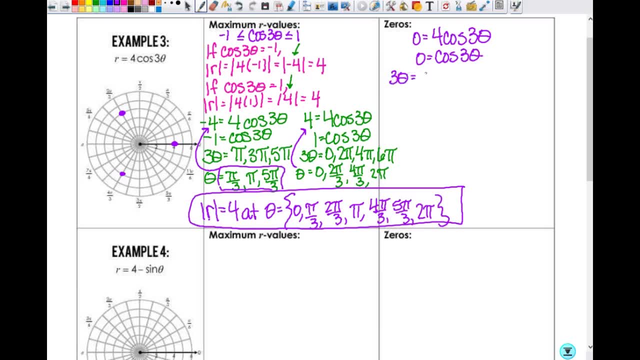 So three theta equals. when is cosine zero? Pi halves, three pi halves. but I'm gonna have to go to six pi here, right? So if you think on the graph here We got, this is pi halves, this is three pi halves. 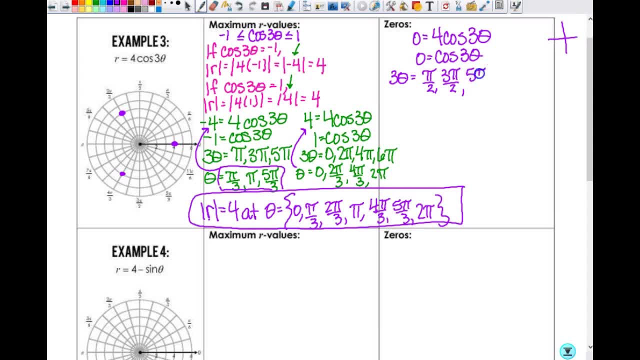 That's four pi halves. this is five pi halves And you know, all those times you did these patterning things and you know had these are my three fractions, what do you think? the next fraction is Same type of thing here. 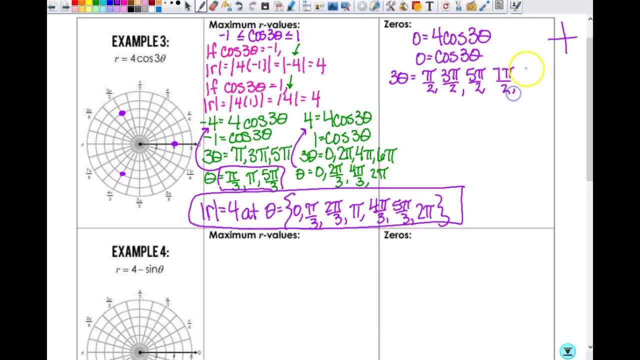 What would the next one be? Seven pi halves, then what Nine pi halves, and then what Eleven pi halves. You see how you're just adding two to the numerator every time. Okay, And eleven pi halves. that would give me here, so then that's twelve pi halves. 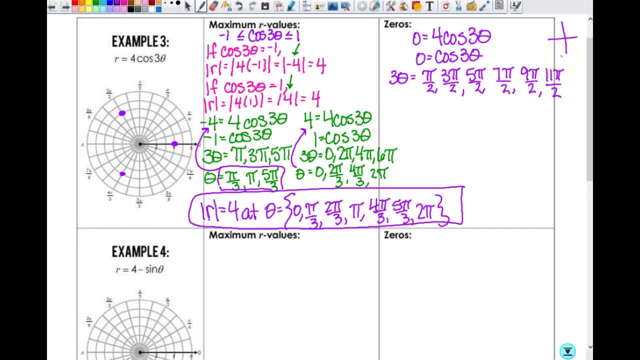 That is three root of six pi. gotta run the six pi, So now I need to get theta. So I'm gonna divide everything through by three. Is that gonna be easy or difficult? Easy: Dividing by three is the same as multiplying by one third. 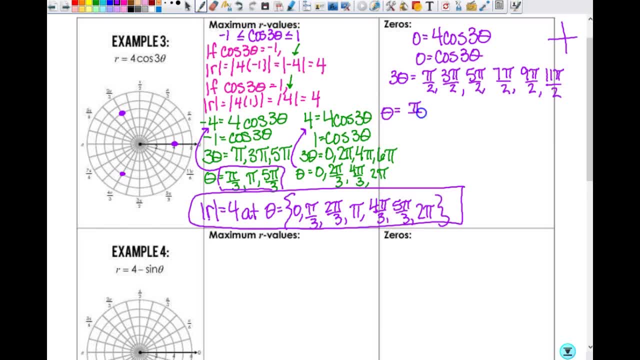 So I get theta equals and that's gonna give me pi six. What is three pi six? Mm-hmm. So it's pi halves, Okay, And then this is gonna be five pi sixths, then seven pi sixths. what would nine pi sixths? 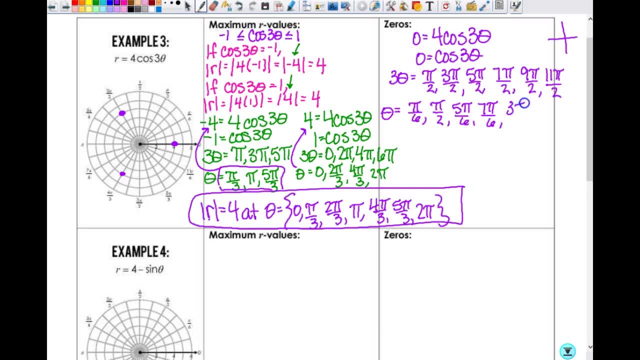 be Three pi Three pi over two, and then eleven pi sixths, right. So instead of rewriting that again, we can say r equals zero at. I'll draw a little arrow in this variance here, because they're already in order. 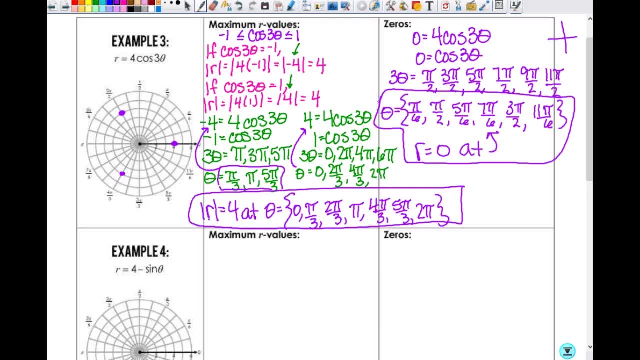 I had to rewrite all these because they weren't in order, but Okay, So now let's think about how that helps me graph this. I start at zero and I'm gonna rotate around to pi sixths. Well, at pi sixths my radius has to be back here at zero. 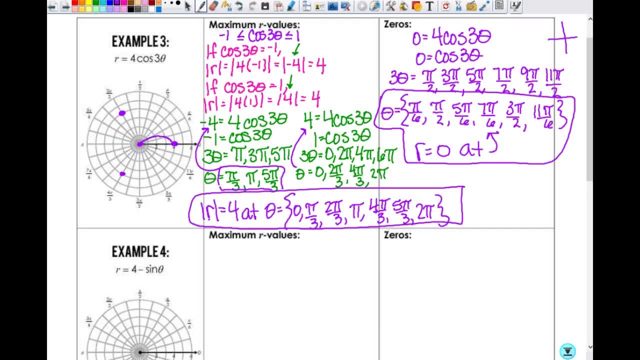 So as I rotate around, it's gotta go like that. Then my next zero is at pi halves and I have a point out here- at two pi thirds. That means I'd have to start at pi halves and come out like that. Then I'm going to five, pi sixths. 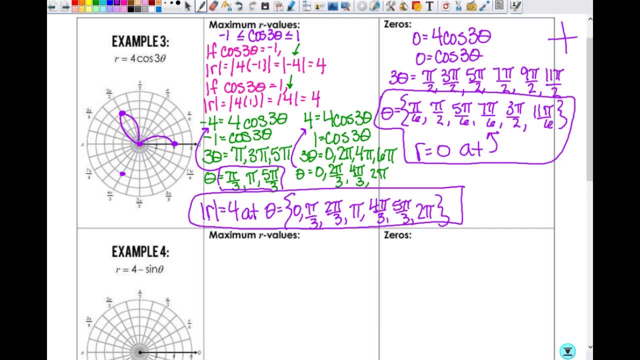 So It would come in like: And then seven pi sixths, so I can't go out any farther than that, can't go out any farther than three pi halves, can't go out any farther than eleven pi sixths, so something like that. 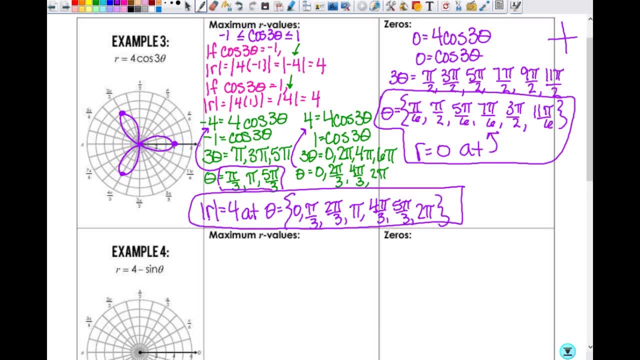 but a whole lot better. So does this have symmetry? if it was drawn better, Yeah, What kind of symmetry? Polar. It has polar axis symmetry and pole symmetry- right, Doesn't it have? Does it have polar axis symmetry? Yes, 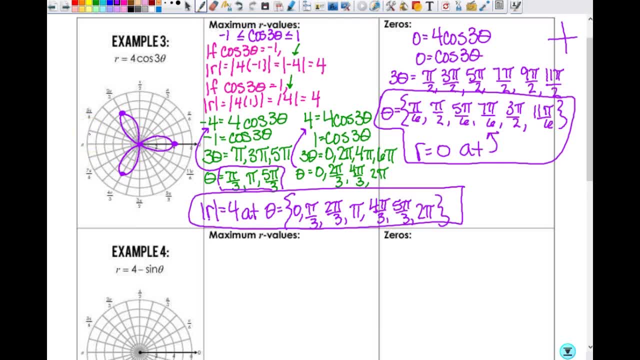 And it has pole symmetry. Does it have pole symmetry? Can I rotate it 180 degrees? No, If I rotate it 180 degrees it's not gonna look the same. I only have polar axis symmetry here. Okay, Does that make sense to you? 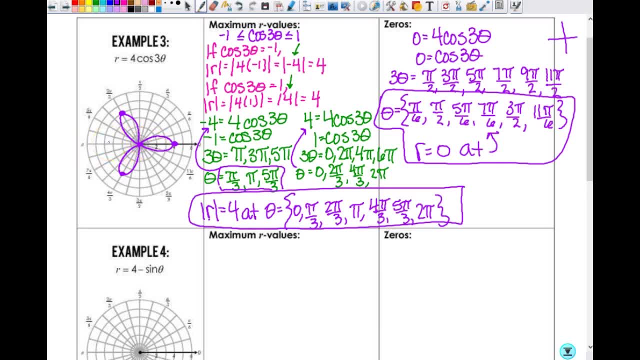 But you will get to where you can look at these and you know it's gonna be a rose with however many petals. so once you can get one of the petals, then you'll know where the other ones are. Plus, if you can get this part of the graph drawn, then you should be able to reflect. 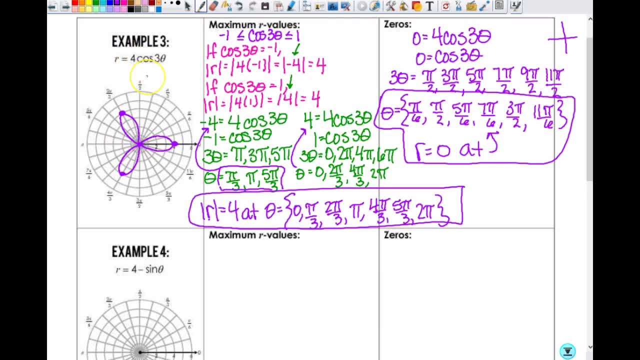 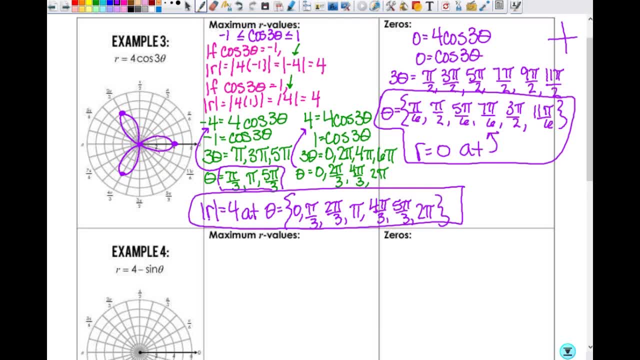 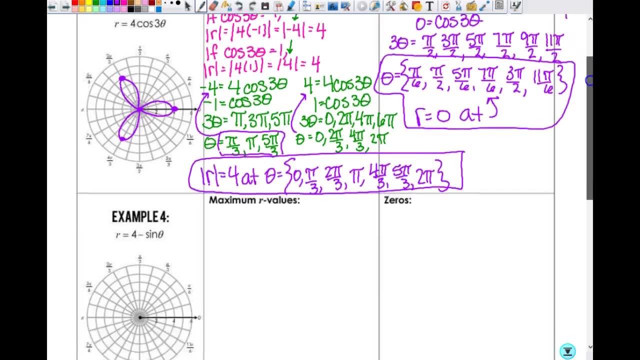 All right, All right, All right, Any questions at all? All right, I'm gonna get you started on the last one, just because it starts a little bit different, and then I'm gonna have you work through it. So we're gonna start with our maximum r values. 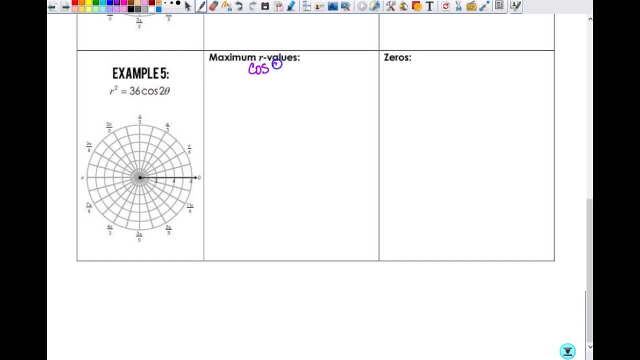 This is 2 pi. so that means that the cosine of 2.. I'm sorry, not 2 pi 2 theta is less than or equal to 1,, greater than or equal to negative 1.. So I say: 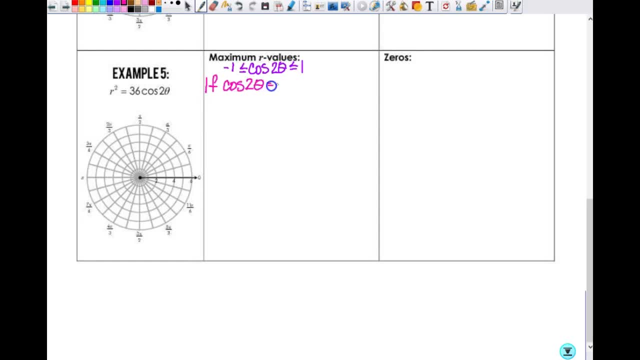 cosine of 2 theta equals negative 1, then the absolute value of R equals. well, this is R squared. so to get R, I'm going to take the square root of both sides right. So it's the absolute value of the square root of 36 times a negative. 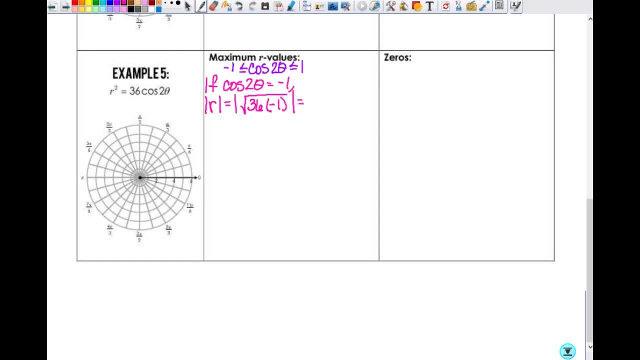 1.. Okay, well, what's the square root of 36 times a negative 1?? It's an imaginary number and we're only concerned with the real numbers right here. so technically this doesn't give us anything. This is the empty set. Empty set looks like a. 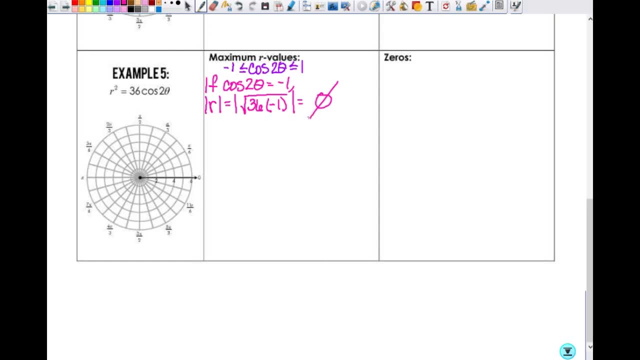 zero with a line through it, So we don't get any answers out of that. You will get answers out of the other one, though it's not another empty set, So go ahead and finish this part up once you get this. start like attempting to graph. 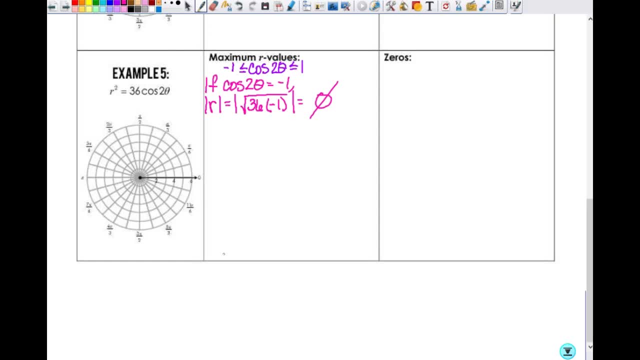 it right: Get your zeros, attempt to graph it. I'll give you some time to get that done. 1., 2., 3., 4., 5., 6., 7., 8., 9.. 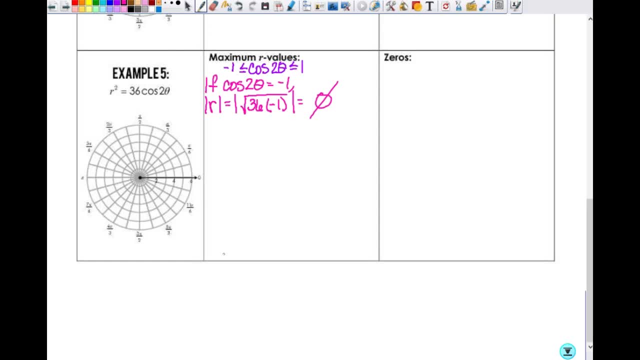 10., 11., 12., 13., 14., 15., 17., 18., 19., 20., 21., 22., 23., 24., 25., 26., 27.. 28., 29. 30., 31., 32., 33., 34., 35., 34. 35., 36., 37., 38., 39., 40., 41., 42.. 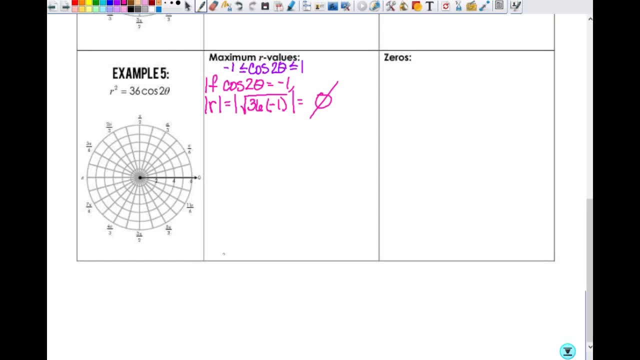 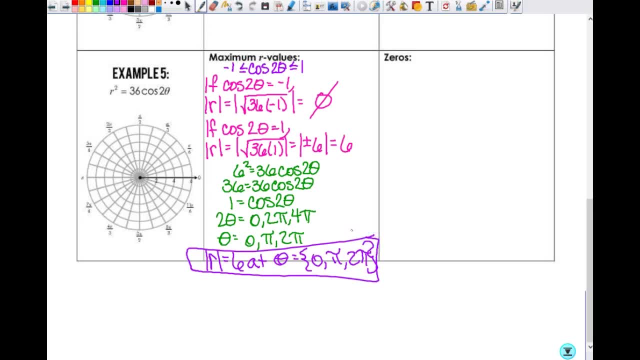 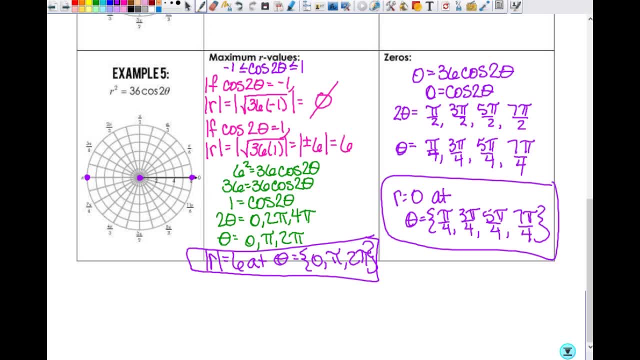 Okay, make sure you attempt the graph. Okay, make sure you attempt the graph. All right, are we ready to talk about the graph? We know we have our radius at 0, pi, 2 pi. We've got a 0 somewhere, right. 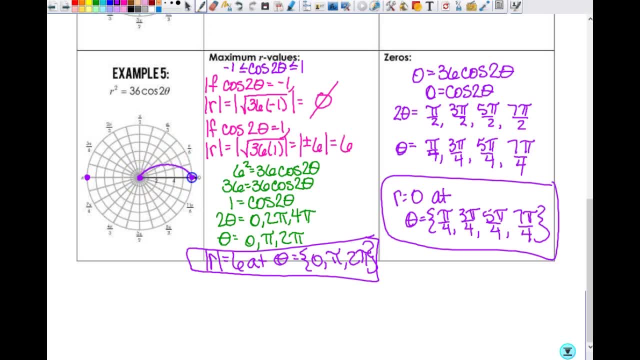 We'll start here. Our first 0 is at pi fourths, so this has got to come out something like that. And then we have another one at 3 pi fourths right here. So this is going to have to come out something like this: 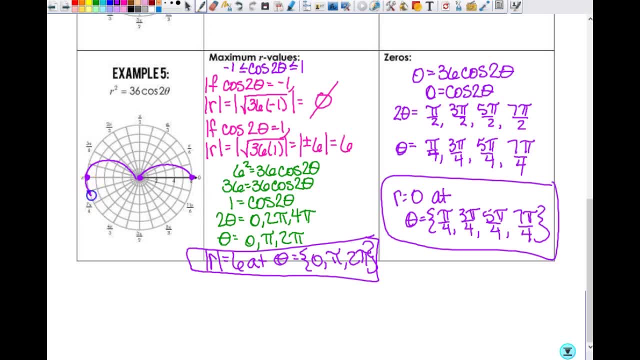 This is actually more like balloony looking than the other one was, but Oh, okay, I can't do it from this side. hang on. Oh, that's still not good, but good enough for now. And they're not pointy, they're curvy. and when you tend to do it in sections, 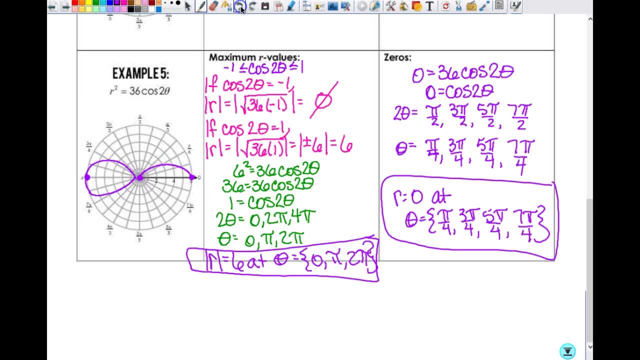 it's like: oh, that's really bad, like really really bad. Let me back up some. See if I can do it better. I have to stand in front of it to get my hit look decent. Okay, that's still not great because it's puffier than that. 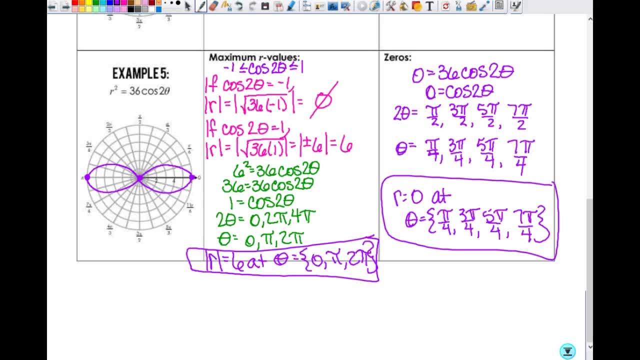 but it's good enough for the talking purposes. What kind of symmetry does this have? Polar axis symmetry, right? Is that pole symmetry? Does that have pi halves symmetry? It has all of them right. So here's why this is important. 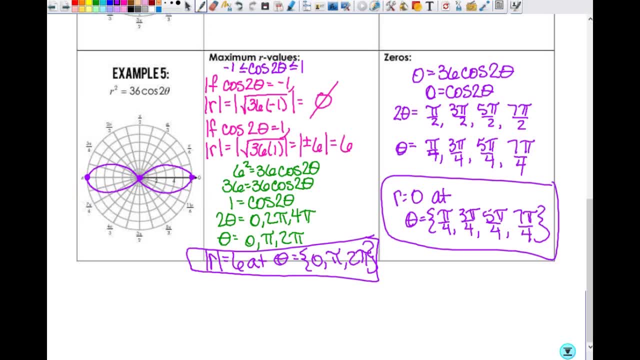 When you actually start applying these graphs and calculus and you have to find the area inside of here, then if you can just find the area of this little piece, then you can do what with it. Multiply it by four right, Or when you're trying to graph it, you can get that. 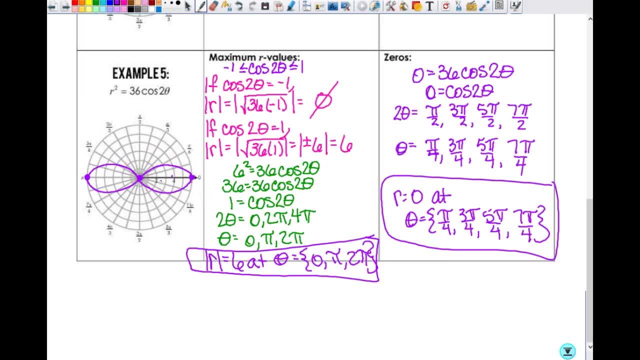 and if you know what it's supposed to look like, you can reflect it and you don't have to go and calculate all that stuff. Okay, does that make sense? So there's reasons that all that stuff is going to be important for us. 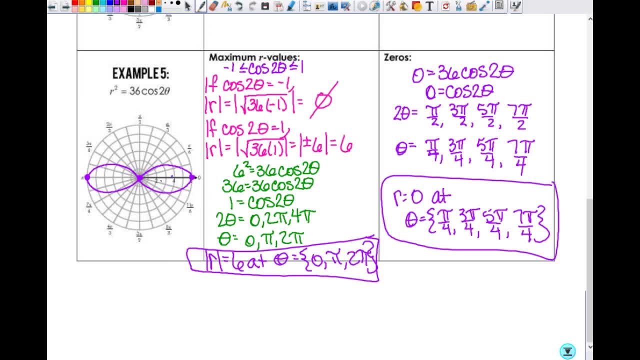 Any questions at all. All right, look at the assignment real quick. It has two sides, One of the sides you're going to ignore. Ignore the side with no graphs, because it's going to be a lot of work. The questions aren't exactly the same.